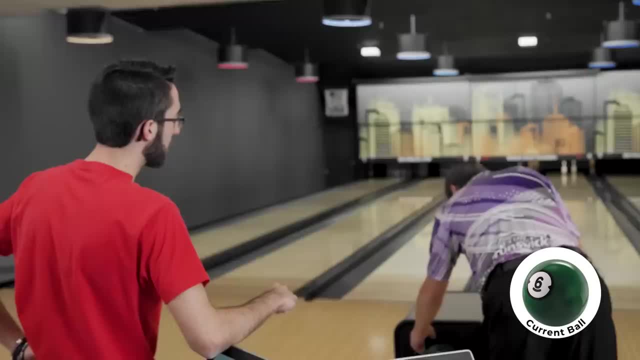 Didn't exactly make this easy on myself, but we got another shot. If you hit the right side of the headfin, I am waiting for the ball to come out of your hand. I am waiting for the ball to go in front of the sixpins. 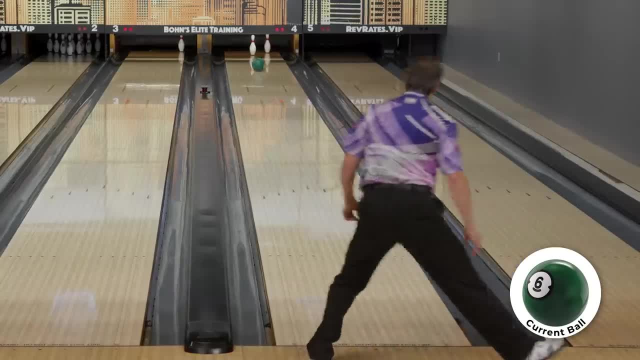 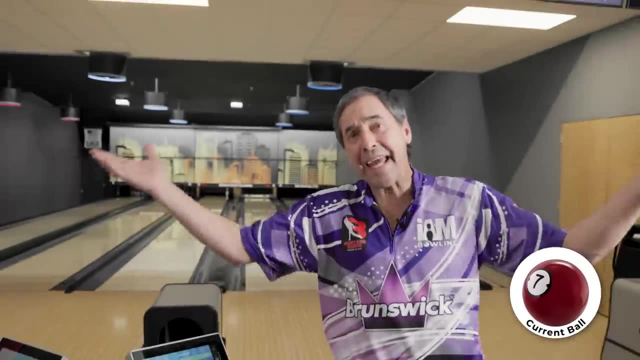 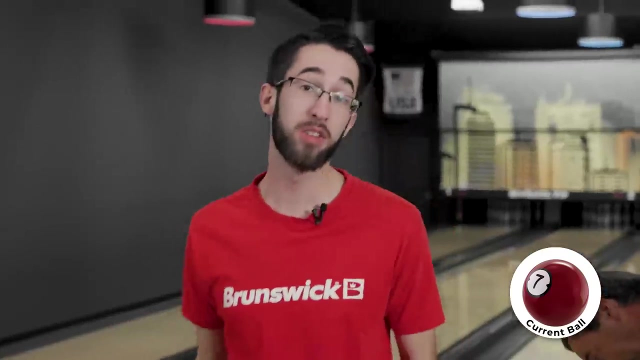 Nah, It might do. it Didn't deflect that much. That's a spare. Any way you shake it, it's a spare. That was a little better than the first frame that I had, because you know I got gutter six. 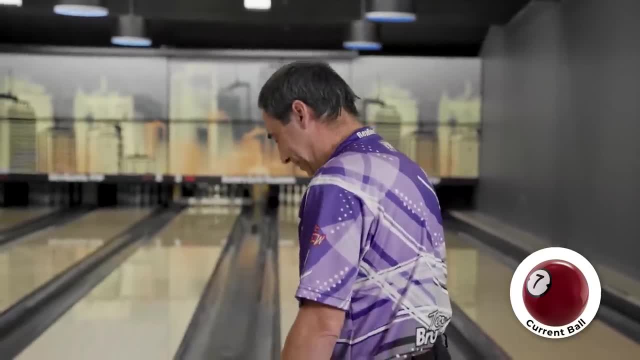 Hey, you're gonna upgrade Your next frame. you get to go to an eight pounder, You're right. So I think, as the game goes on, the pin counts are gonna get a little bit better because we're throwing balls that are heavier, that are gonna go to the pins a little bit. 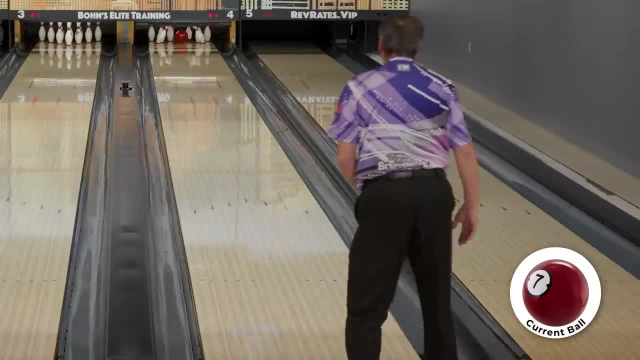 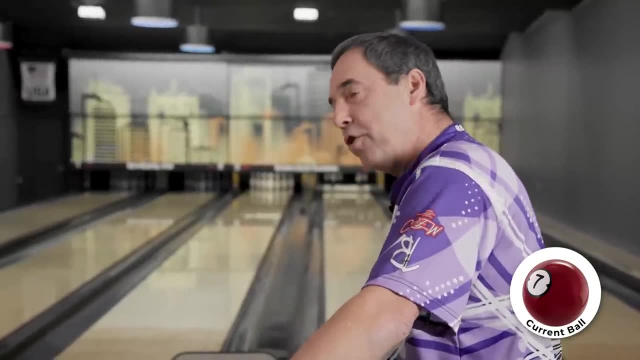 better. You know every frame adding a pound to each ball. I cannot believe your ball went through it. that good to Greek church Five, Yeah, But if you notice as the ball hits the pins, it's definitely slow motion. 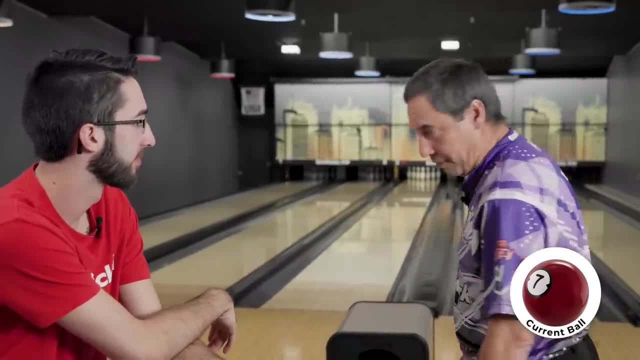 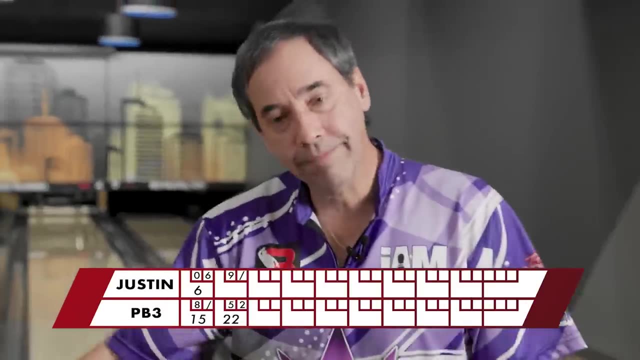 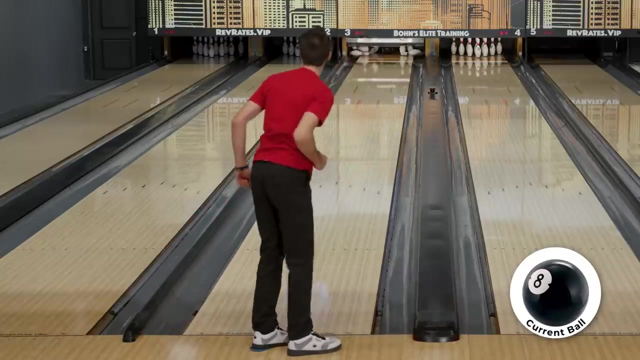 Yeah, Take notice of that, everybody, as we get further along in this game. Yeah, Yeah, Yeah, Yeah, Yeah, Yeah, I'll take my two and move along. All right, Let's throw this one one-handed, because I can get my thumb in this one now. 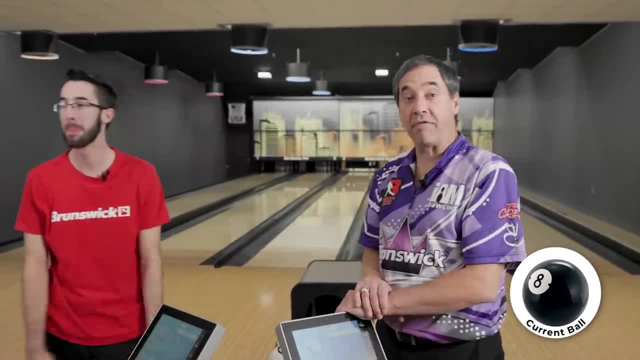 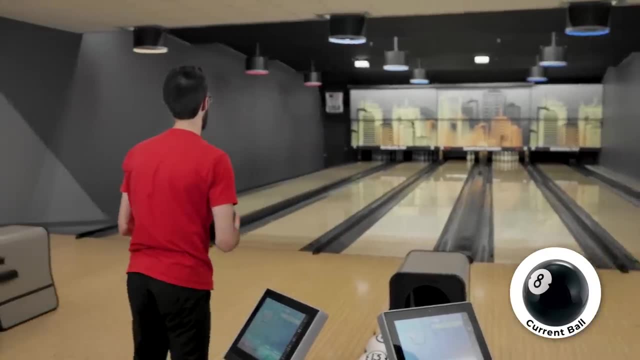 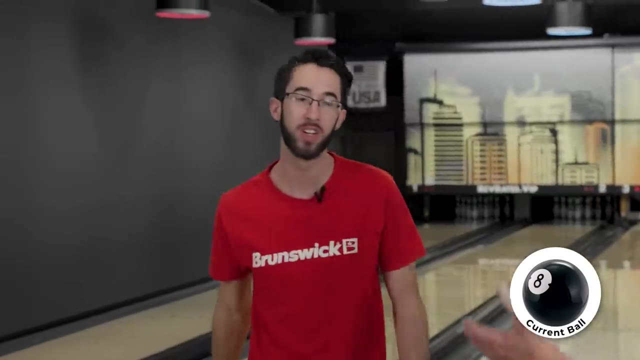 Okay, So through two frames, the six and seven pound balls, no strikes, two spares. Oh, Let's stay tuned. Well, I gotta make this spare. Now you're putting pressure on me. Uh-oh, Saw a hook earlier there, Almost went right past him. 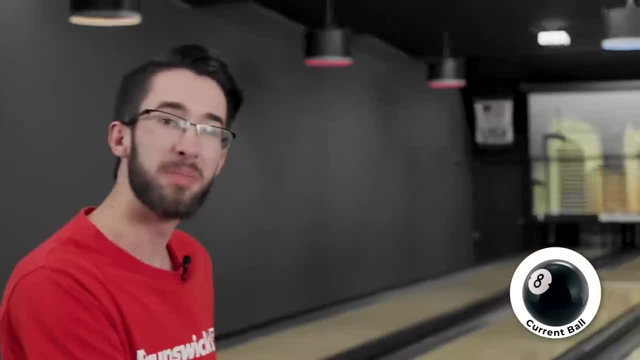 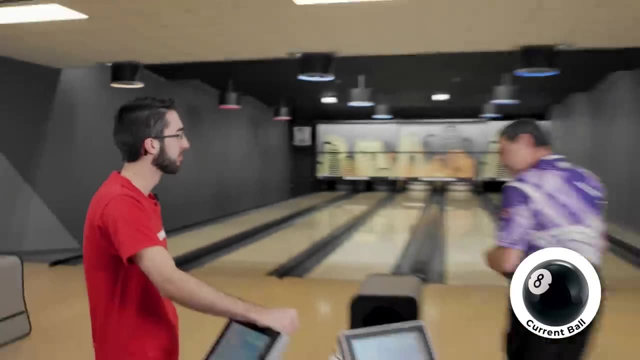 Glad it didn't, Glad it didn't. We gotta beat him every chance we get. So I feel like I got this one right in the bag, All right Off the bat, Right in the bag. You got your thumb in there. 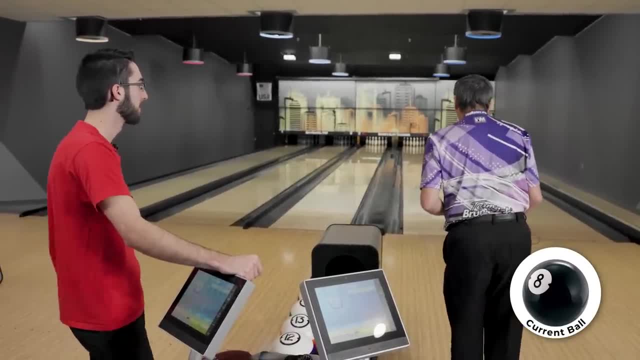 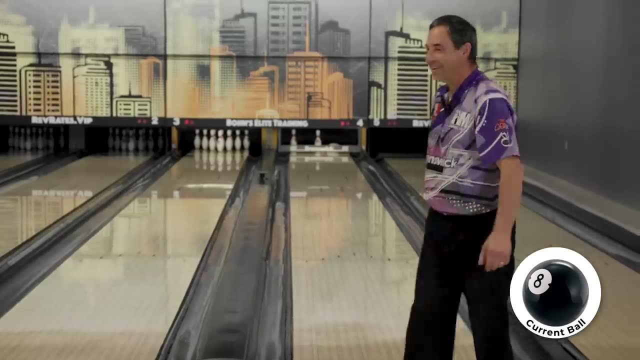 I don't use my thumb anymore, so it's pretty small. You're right. Yeah, This ought to be interesting. Good luck, Oh, close, Close, As the ball hits the one in the front and completely deflects off of it. 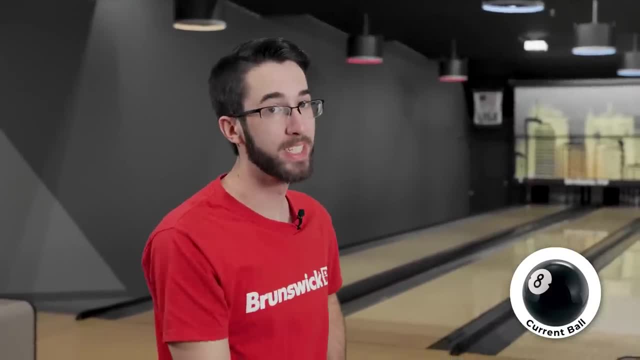 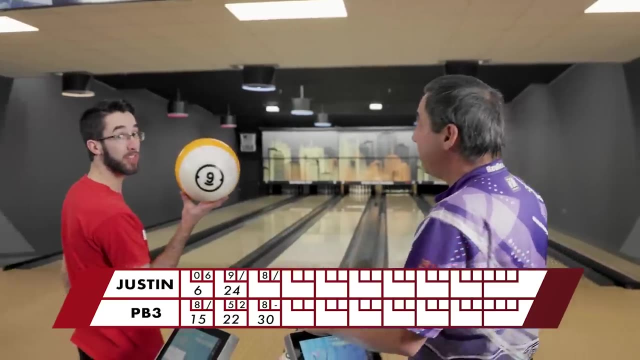 You know, with these light bowling balls, the deflection, The deflection is real. You know, threw it pretty good, Hits a one-two and got no break at all. Upgrade to the nine-pounder here, Going up another pound. 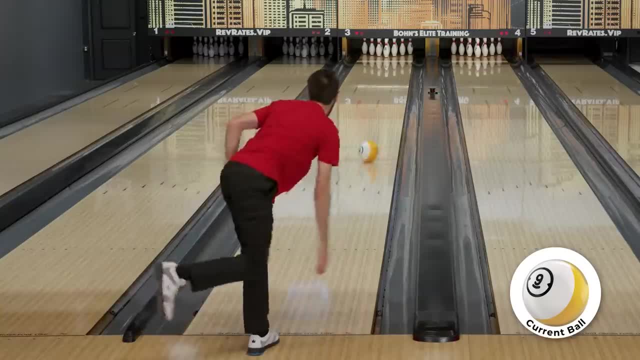 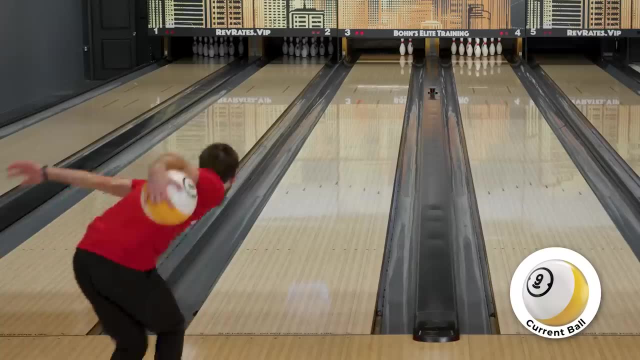 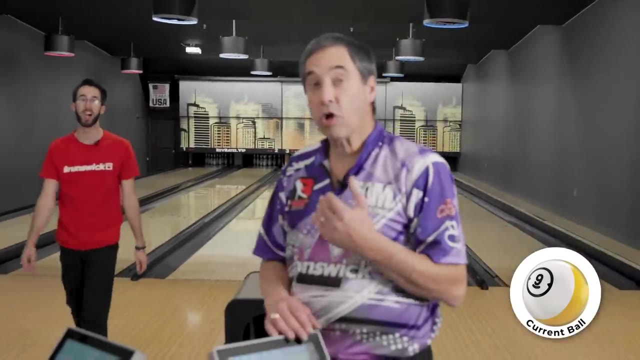 Still not a strike. That was close. That was close. That was close, sir, That was close. Uh-oh, Maybe it would have helped Now if you took close notice there. he did hit it, But unfortunately it did not fall. 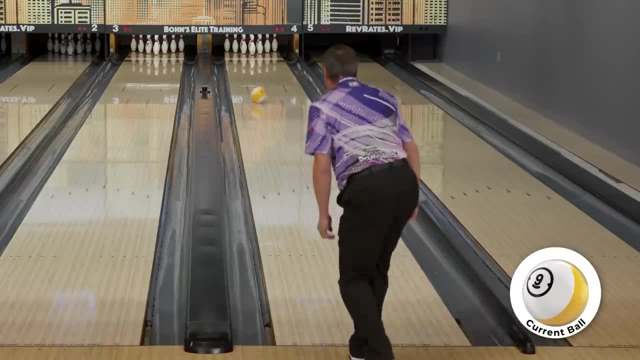 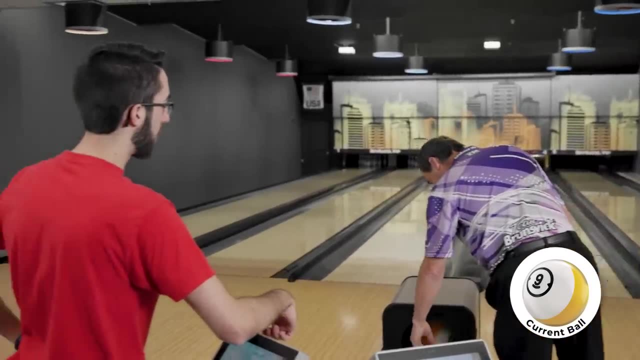 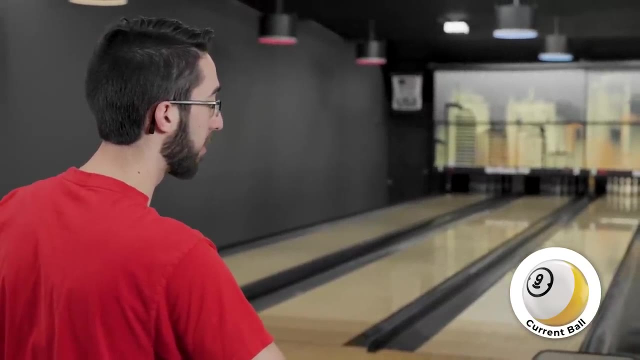 Miss Got nine. I feel like I got an upgrade. You know, I feel like I've watched you give lessons or do shows or clinics somewhere And you do the same thing one finger in the ball, And so how easy it is to make a seven-pin with one hand. 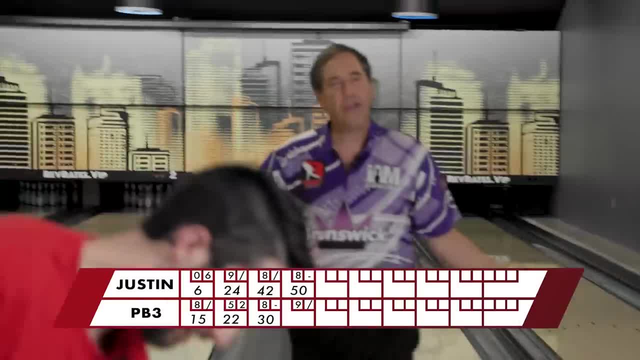 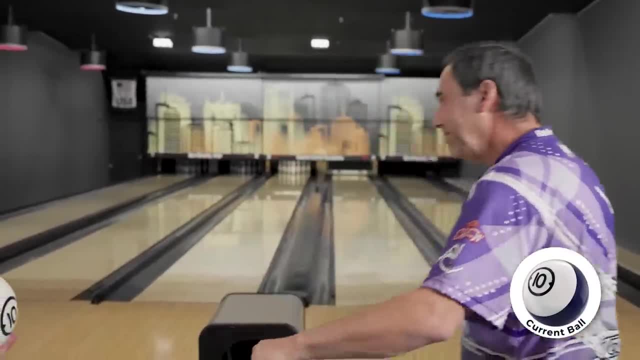 A seven-pin with one finger. All you have to do is knock it over. It doesn't have to be fancy, It just needs to be effective. It's like he's done that a hundred times before. Maybe you should jump on board. 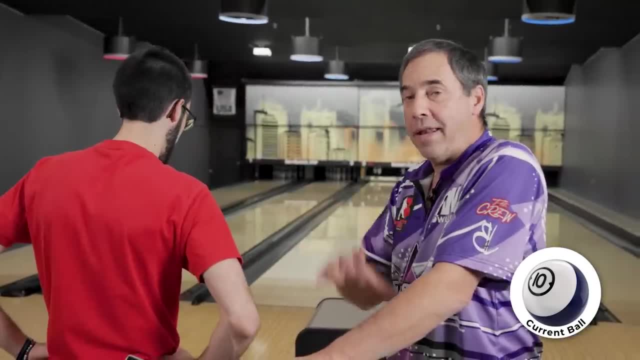 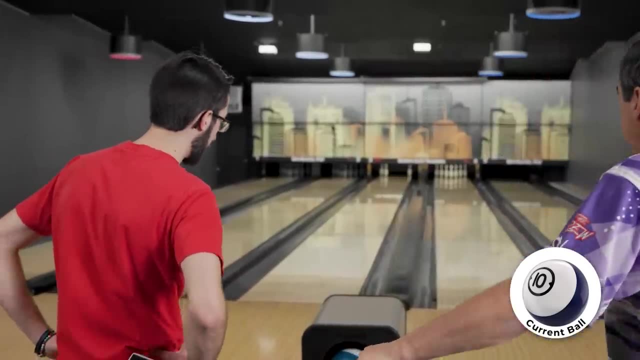 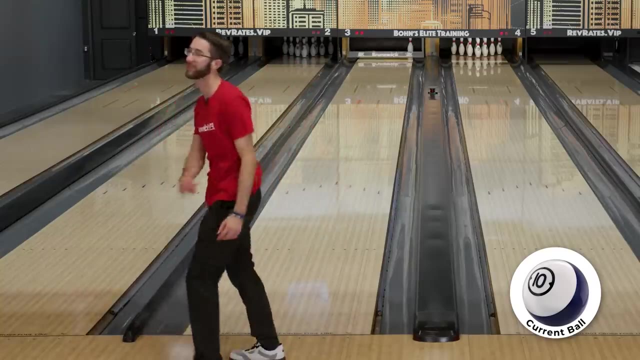 So we are now up to ten pounds. We've got nine shots between us and still not a strike. I think I'm going to put my left hand on it after this one, But for now thumb's going in it one-handed, Both for no cigar. 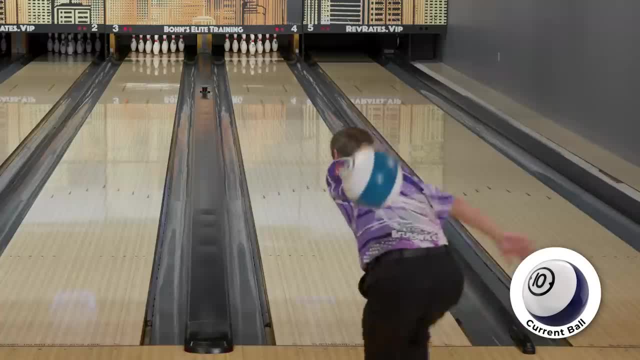 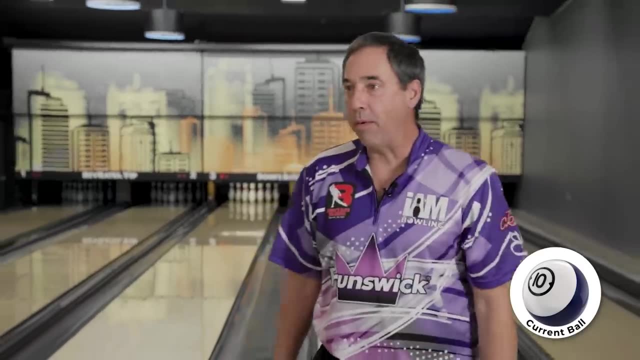 The door has opened. Oh my Oh, that was close. Ooh, The thumb didn't exactly come out of that one. No, And you know this is not exactly going to be the easiest one. No, I was just about to say that too. 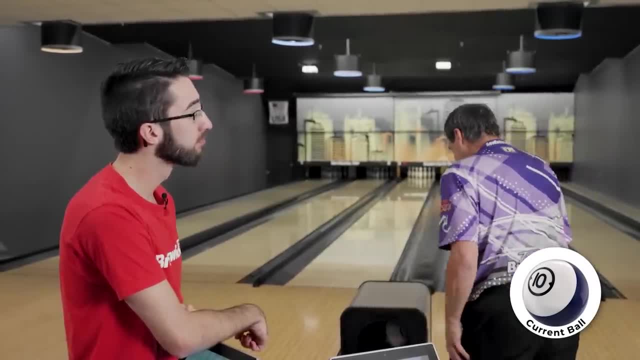 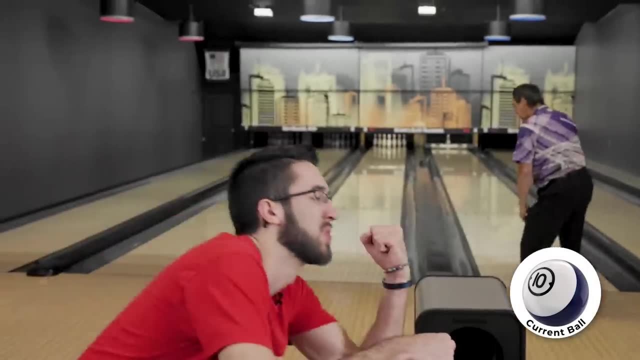 But I'm going to hook it. No thumb this time, Good luck. Oh, Oh man, That sucks. What's the score here? Oh, got the lead. Look at that. Five frames in- Still no strikes. But heavier balls are about to start. 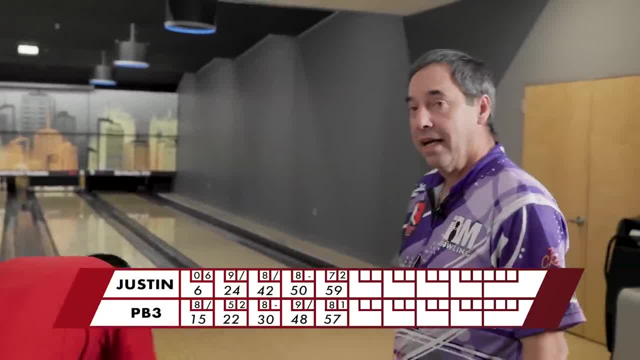 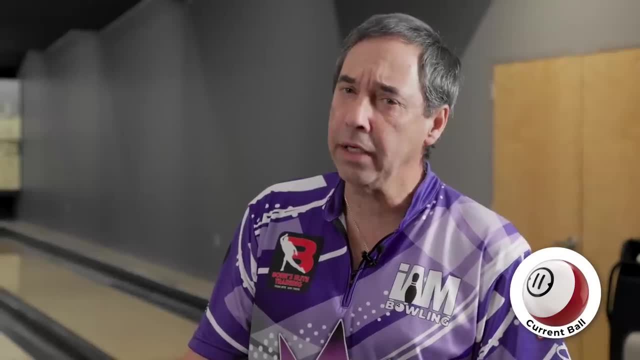 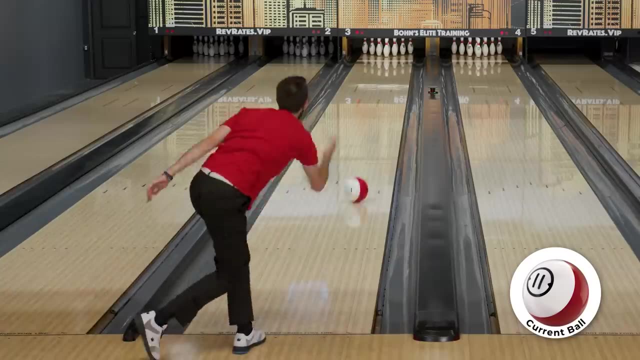 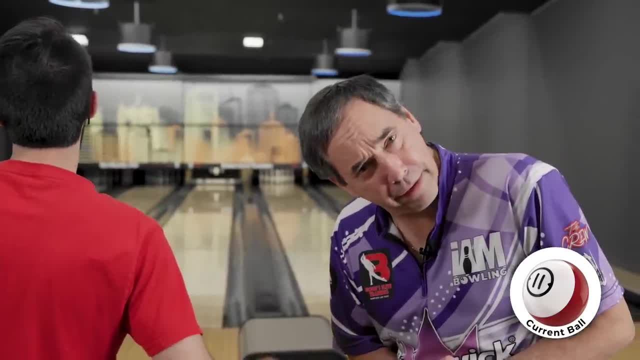 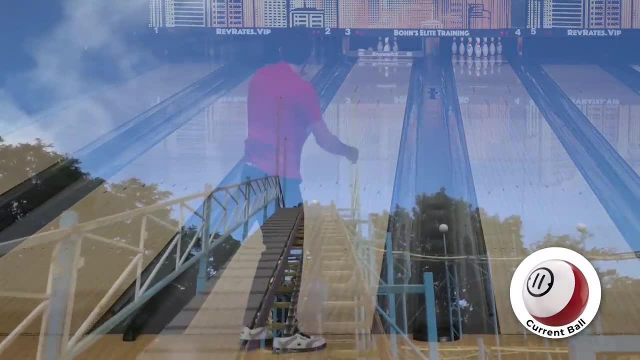 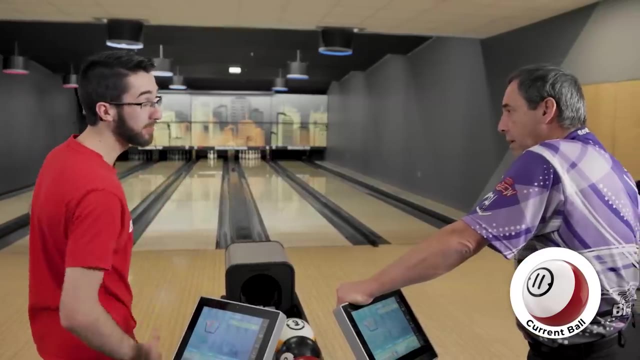 That sounded awful. It sounded like a rollercoaster ride, rolling thunder. Have you heard of that? Wow, Hey, this is the everyday. leave here. You got another hand you want to put on it. No, No, No, The everyday. 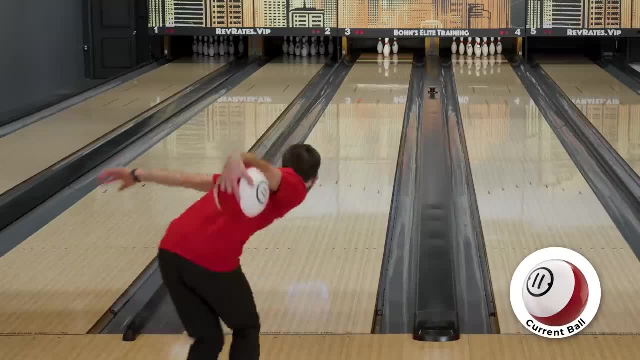 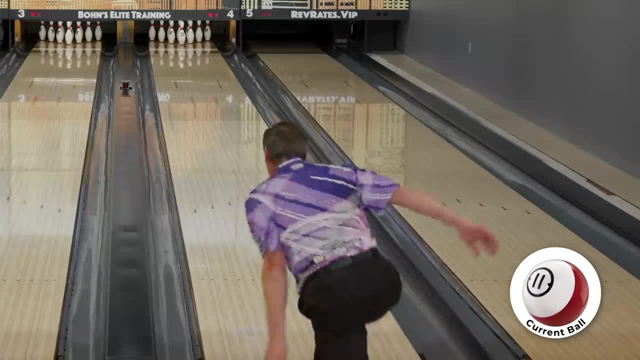 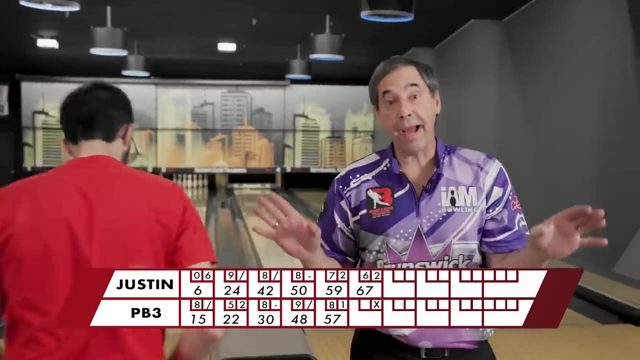 1589 here. Yeah, Leave this one all the time, Not 00.. you know he's saying these weights are gonna get good somewhere. I better hope it starts coming. I guess it started for him. you know it was not pretty by any means, but from the average bowler, 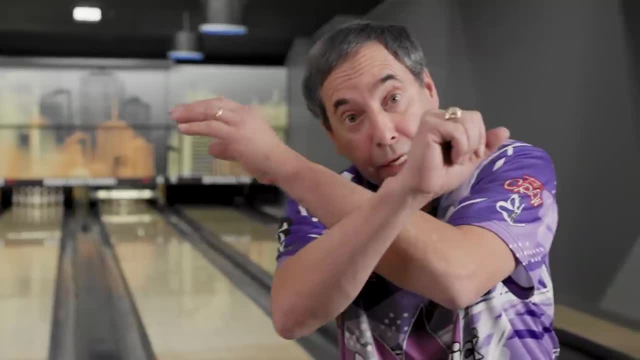 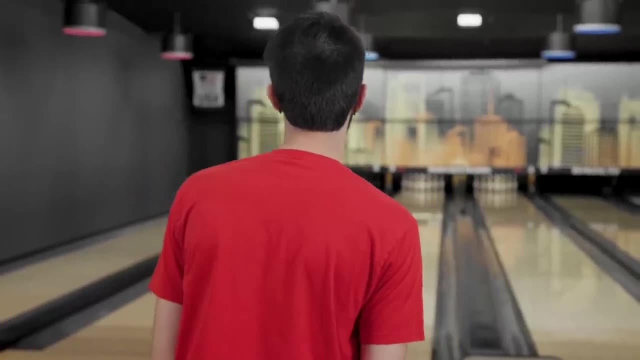 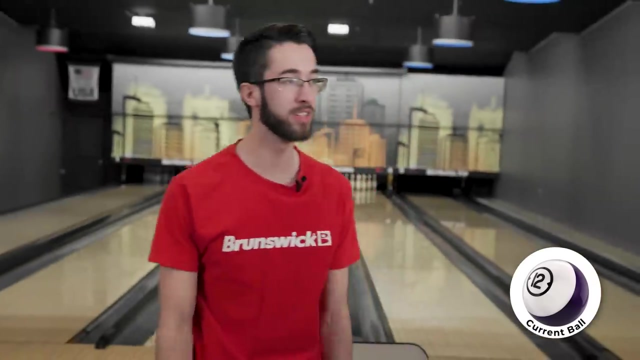 right now. I'm glad they all fell down, so I think I'm gonna try to stop doing something fancy here and just try to hit the one in the front. nice and easy, as they say, hit them thin and watch them spin. I hit them pretty thin, watch some of them stay, just not all. so if you notice the ball, 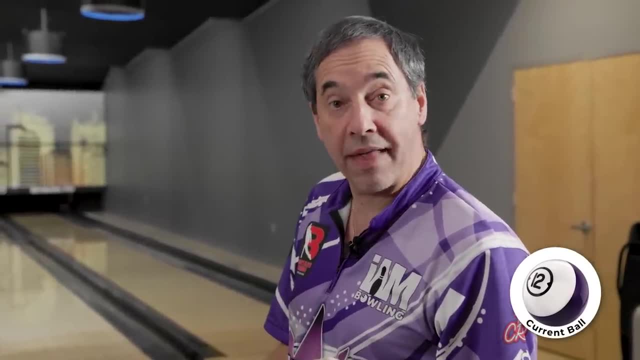 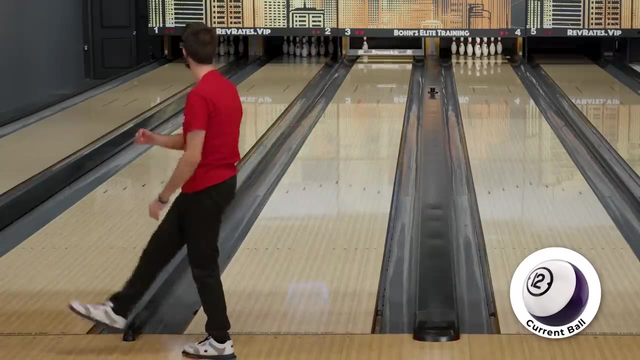 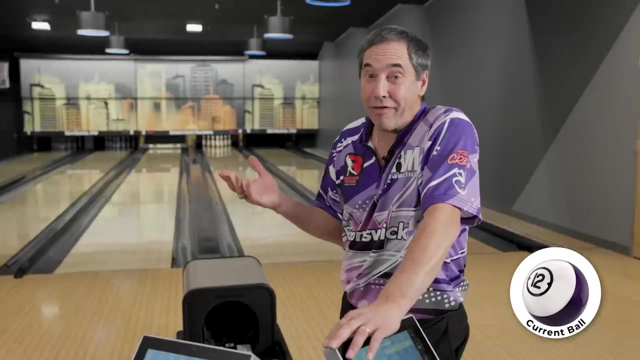 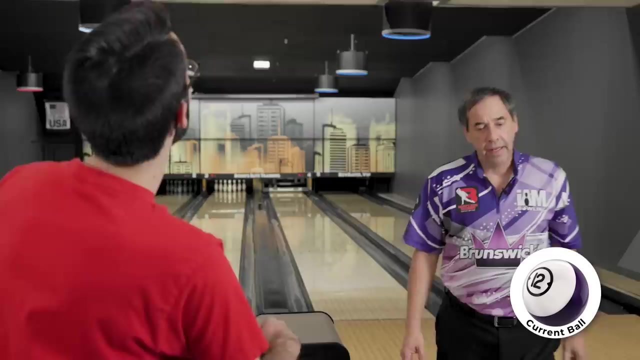 as we get heavier in weight, it appears that they actually go through the pins a little bit more effective. doesn't matter what ball you throw down the lane, it's still the same game. you don't knock it over. the scoring machine gives you a miss. it was high, it went through the nose, but the ball went completely through the pins. 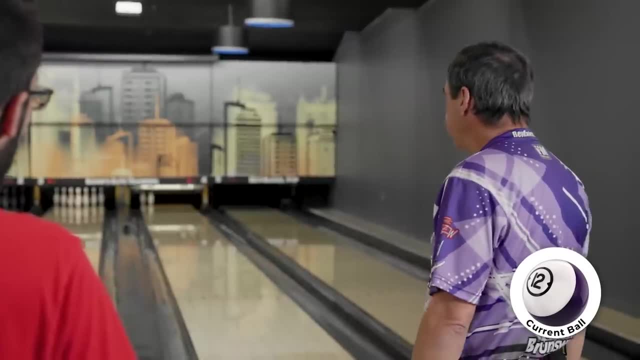 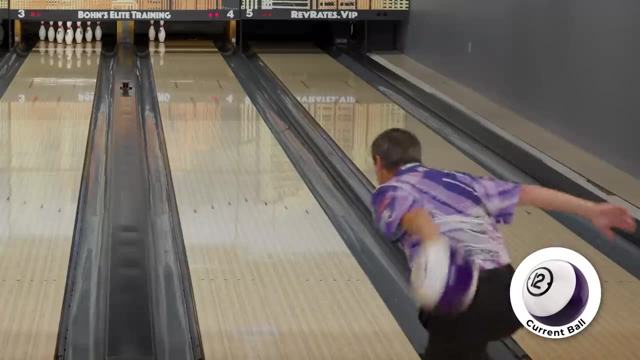 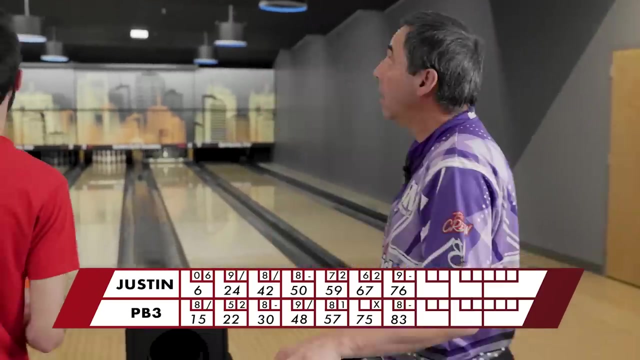 I'm gonna try to make the spare. really, I'm thinking I'm feeling pretty good right now. have you had frames that you've tried not to make this turn? nope, oh no. well, just because you try doesn't mean you're gonna make it. by the way, I am in the lead. you got three frames to go. 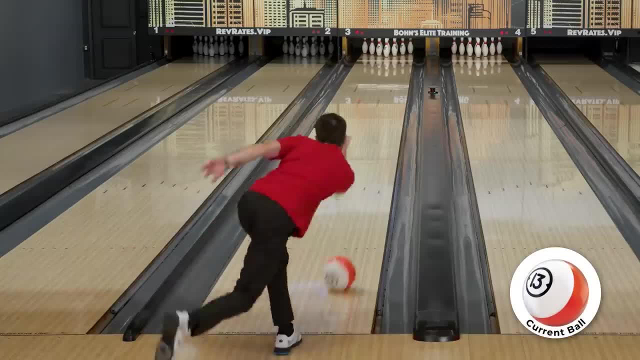 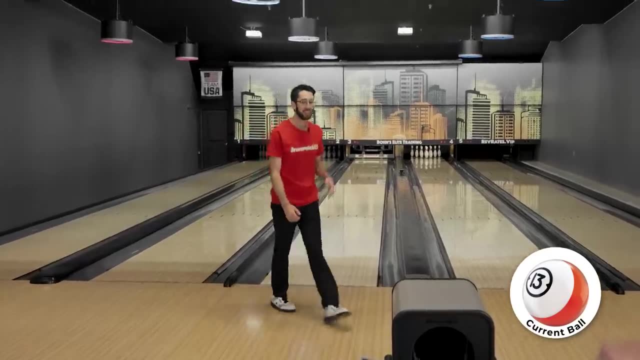 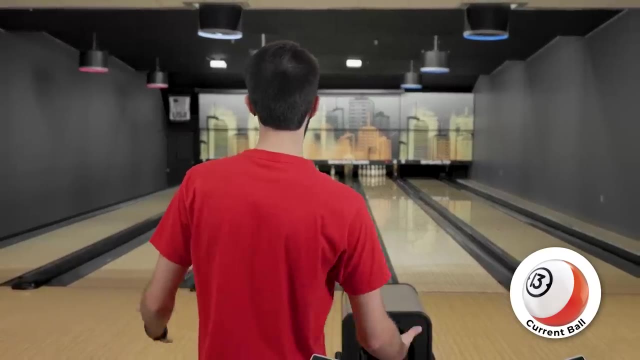 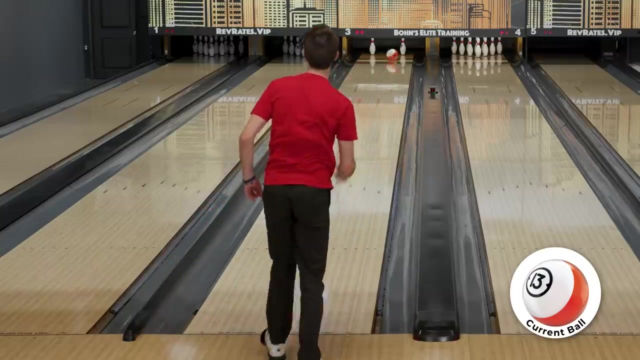 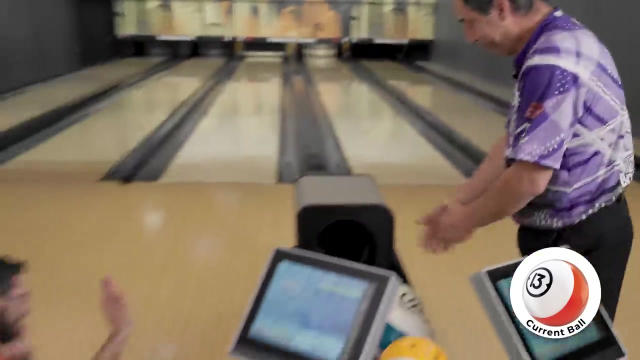 we're not exactly blistering them right now. so you come on, I gotta get a hit somewhere here. whoa man, you leave something makeable, you miss the spare, you throw a good, you split. can we just get a break? that was really a great shot, fantastic, go, go, go again. wrong sport, go again. 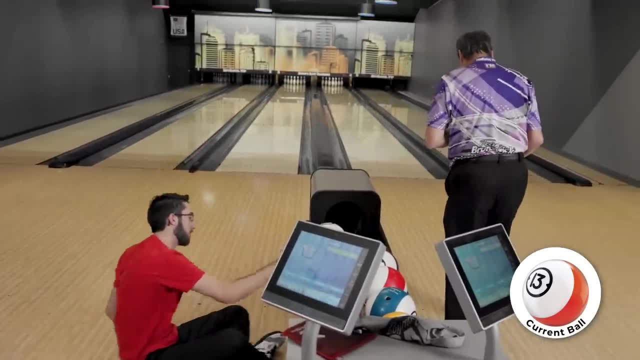 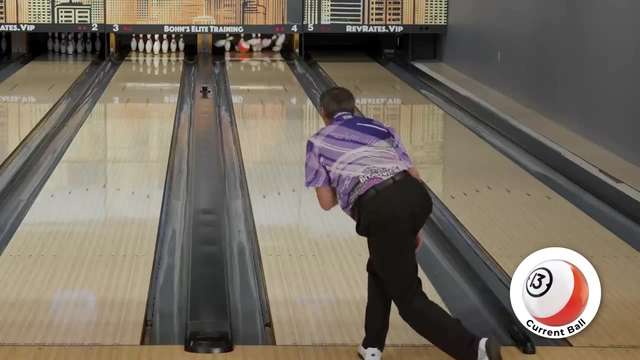 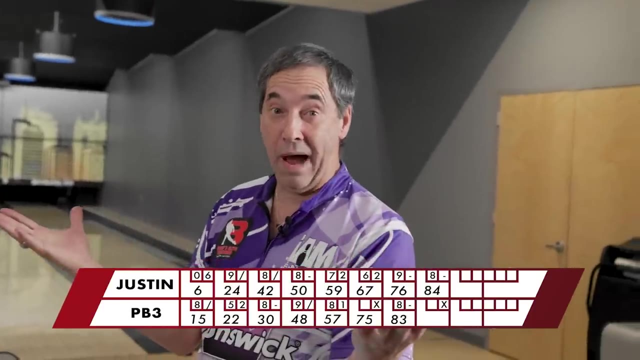 I'm gonna talk to this 14 pounder while you you're up, we'll do 13.. you know you got a lot of work next frame. we better. we got a lot more work to do next frame, so we really better do it. did you feel the power on that one? that was a great shot. I'm gonna go with the, the first. 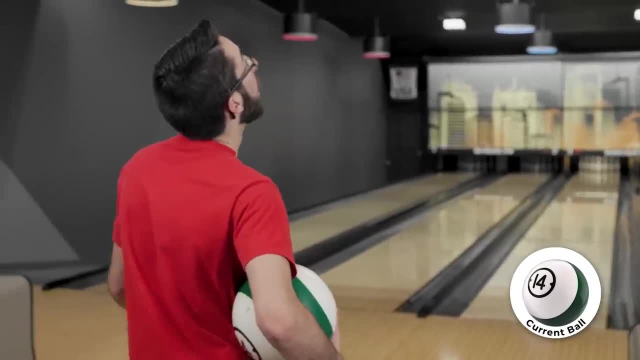 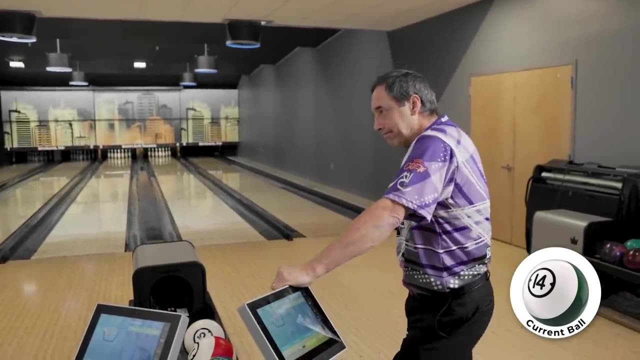 frame strategy. go with the backup ball from the left. you could try to go with anything you want to go, but we're down to only two frames and you keep faltering more behind. I know I'm gonna just uh get Patrick out of the bag here, hopefully. 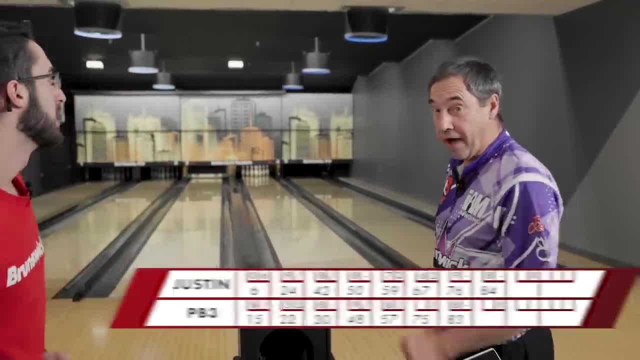 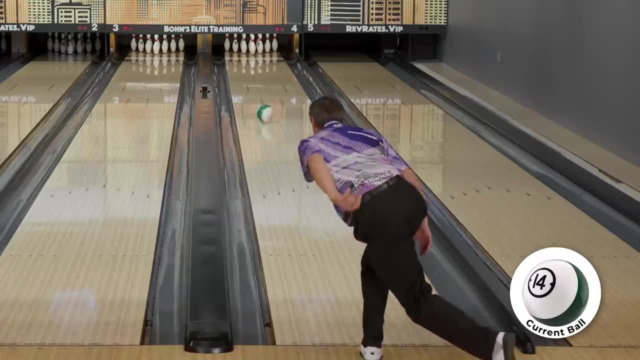 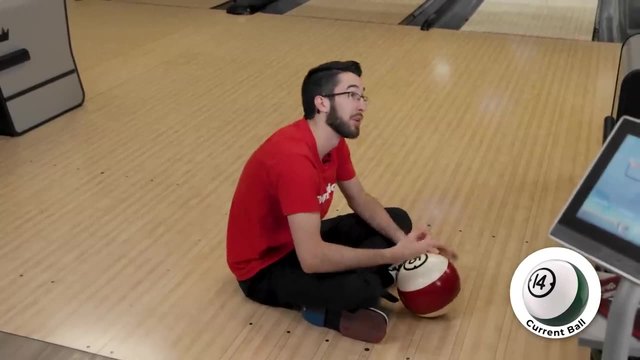 it wasn't pretty, but once again the heavier ball was a little more effective. come on, give me one. make him earn it, as I'm down 20.. could have got a little break there. drip the six out. what are you doing? I'm talking to it if you. 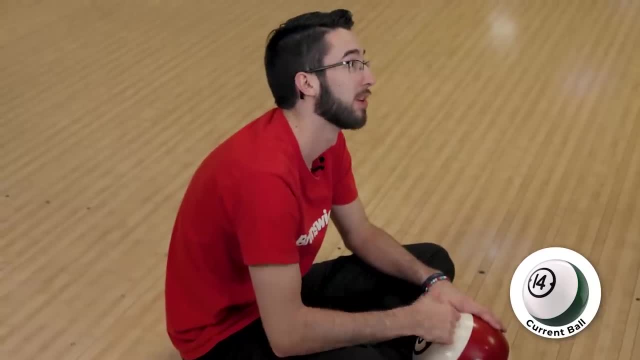 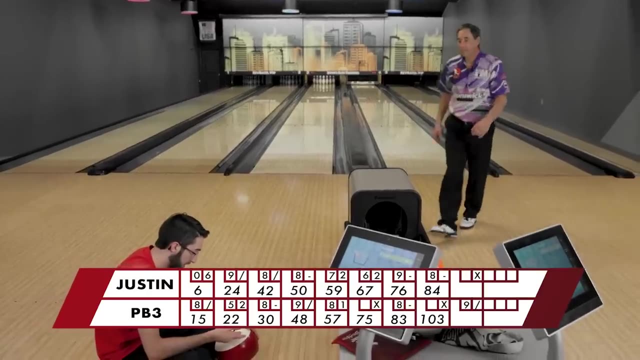 talk to it. it strikes me really. I talked to it last frame in his truck and that was the first strike I had. all game all right, good. but you know, I just had the same conversation with the 14 hound. um, a strike here would be really nice and we, we better do it, okay. so let's do it. teamwork fist. 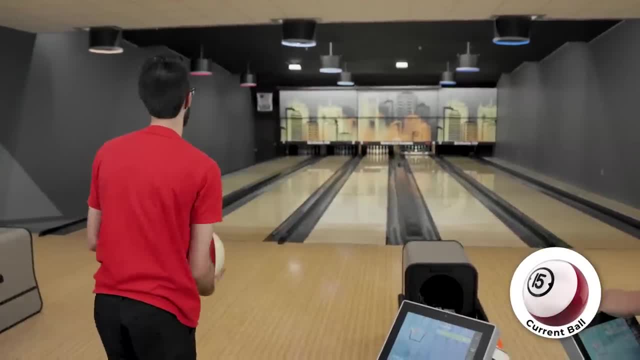 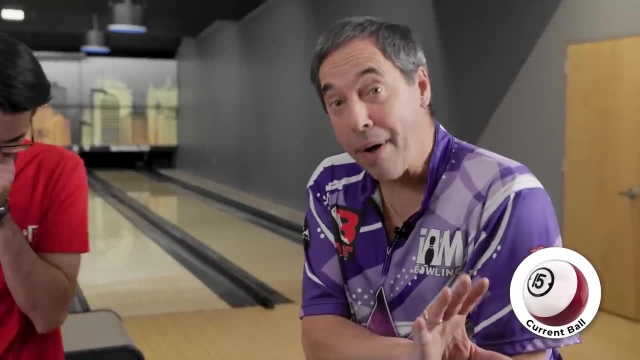 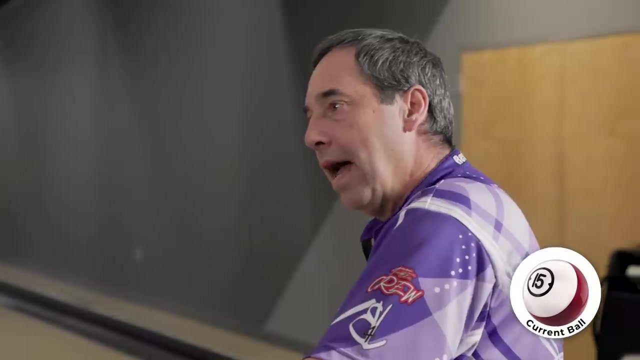 pump. let's do it all right. I talked, gave him the pep talk, we're all good here. oh God, dead. dropped it. and then that popular number shows up once again. don't even say it, thanks. had to give it a long six, extended six, 10 frames, six. 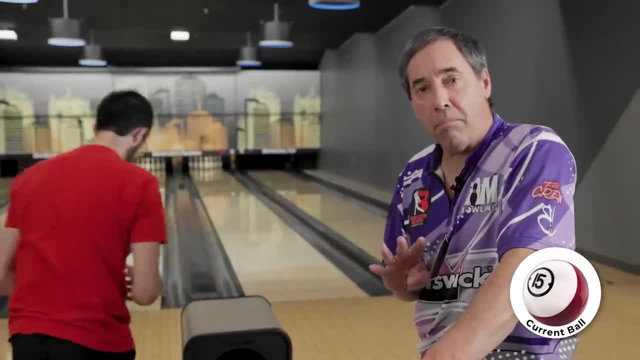 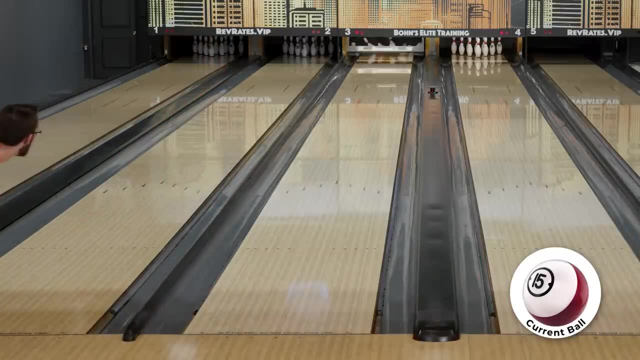 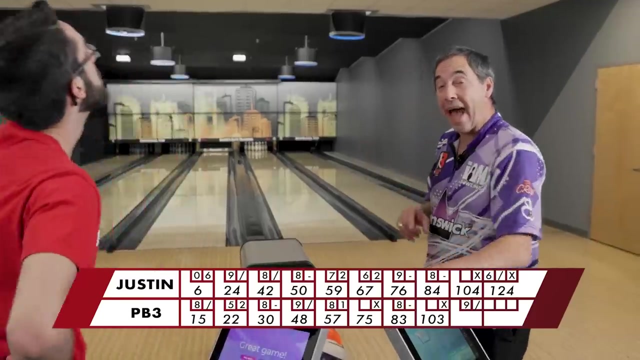 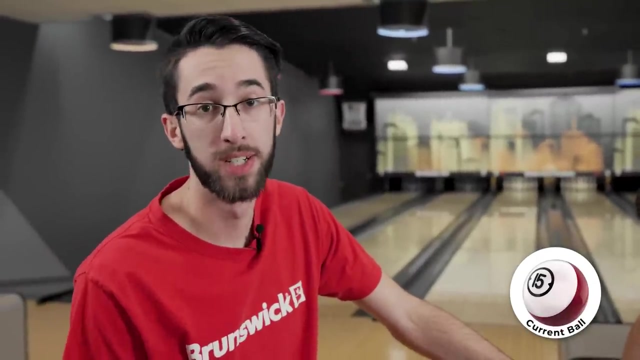 so with the lighter weight balls we had four complete marks spare or strike in the first five frames, ah, and on a strike so far in the back five frames. with the heavier balls we have at least double that bonus tip for you guys. so if you're running the same issue that I ran into, you know where the holes don't fit you. 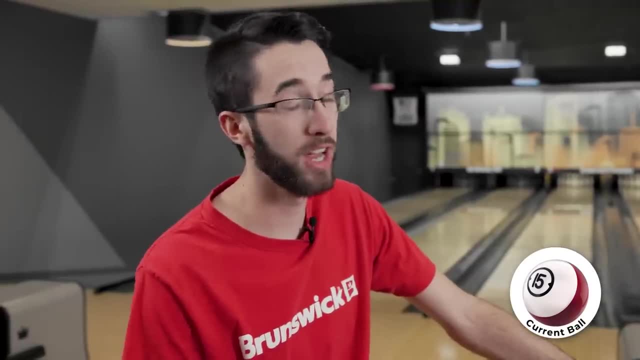 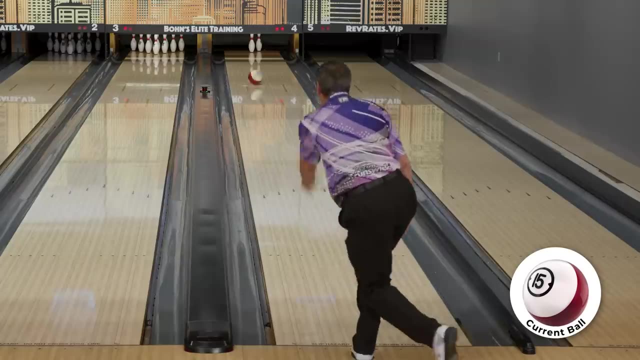 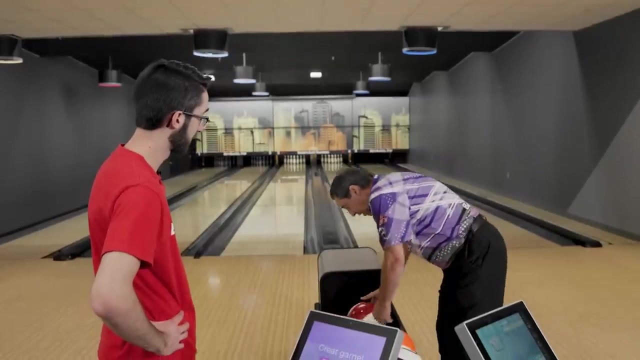 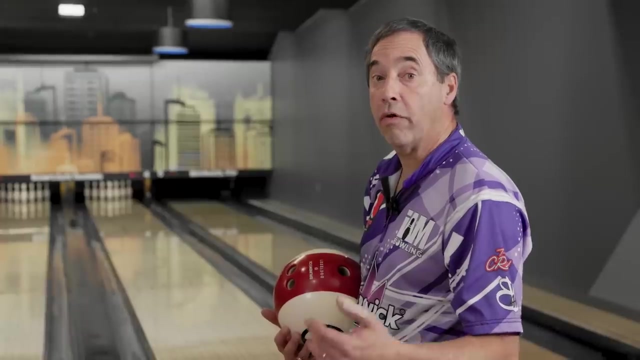 can't go to your local Pro shop and get a ball that fits. you get that ball, you know, adjusted, nice for your hand, safe. do you get them both? of course, it's called the spare. so what's the lesson here today? the heavier ball is more effective, but you throw a weight that really works well for you. you don't.